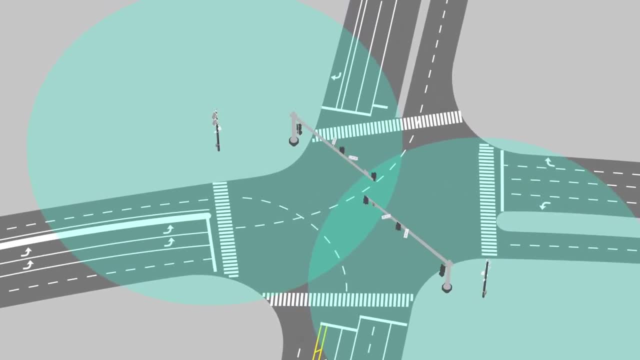 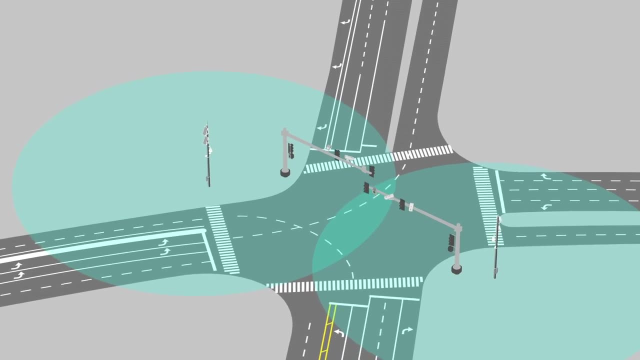 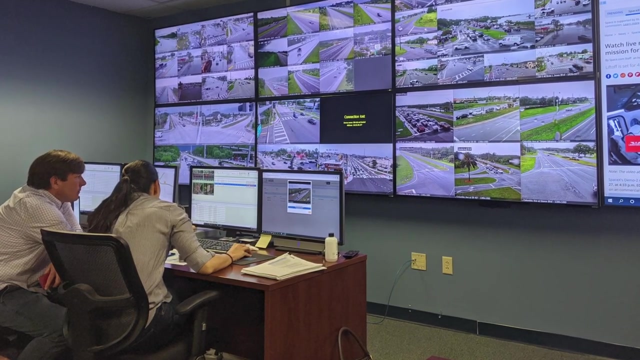 and check the speed of vehicles entering and exiting the roadway. The traffic management center now not only sees the intersection, but has much deeper traffic flow data to use for safety and roadway improvements. Speaking of traffic management centers, our new traffic management center is being envisioned as we speak. 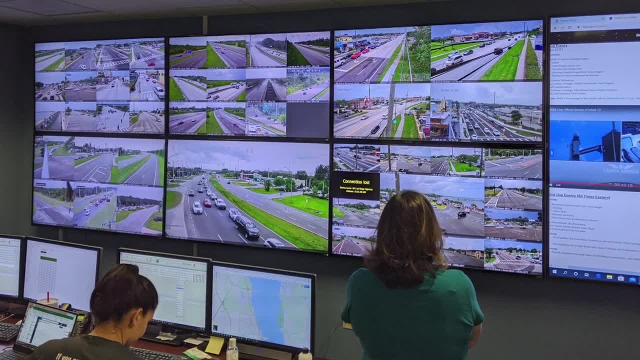 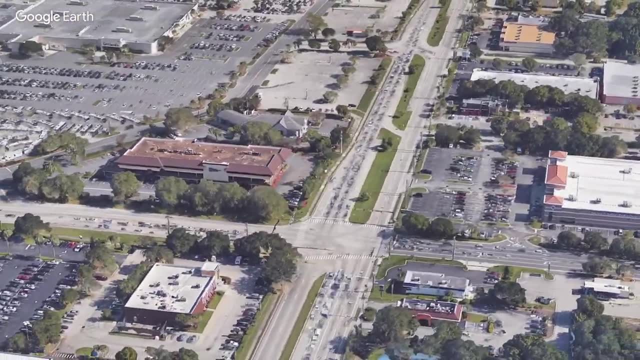 We're really excited about it. It's the brains of this entire operation, after all. Let's travel to another location and look at some more future possibilities. This is the intersection of US and Canada. It's the intersection of US 192 and Hollywood Boulevard. 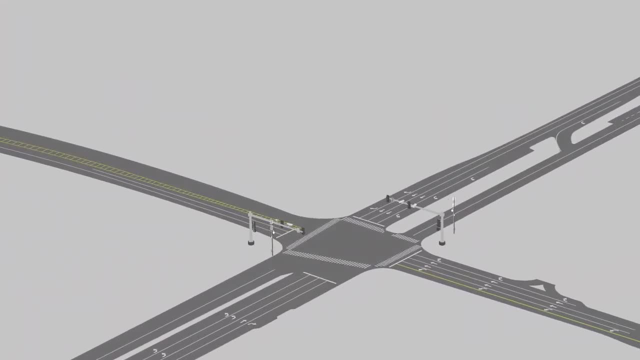 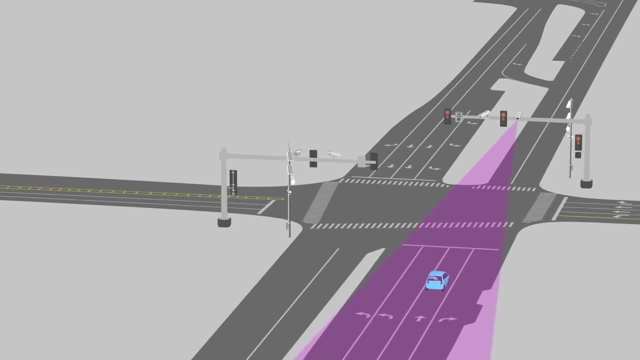 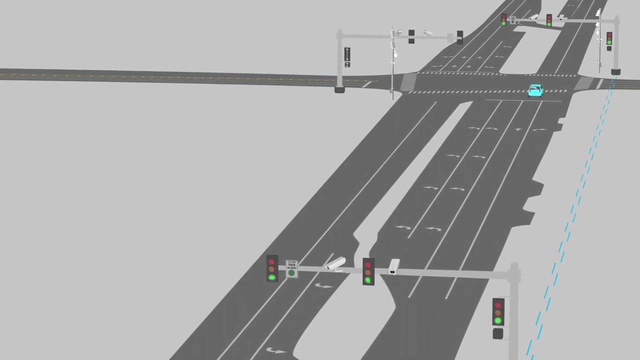 In addition to the technologies we've already seen, this intersection employs another modern technology called signal coordination. Signal coordination uses the vehicle detection sensors to allow other intersections, upstream and downstream, to communicate with each other and work together to predict traffic flow and adjust the signals. 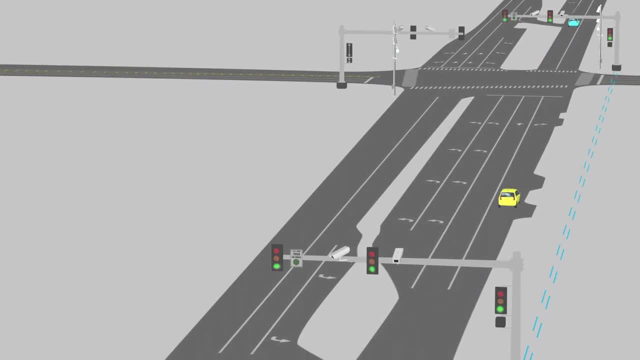 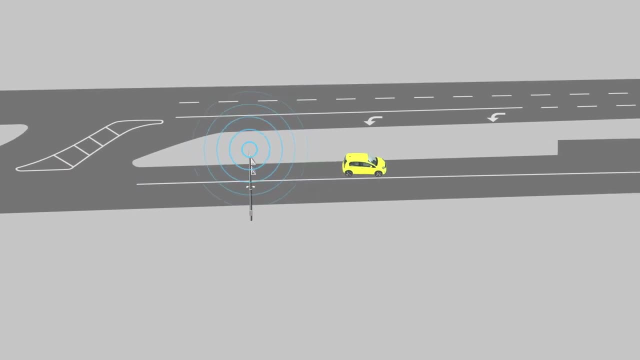 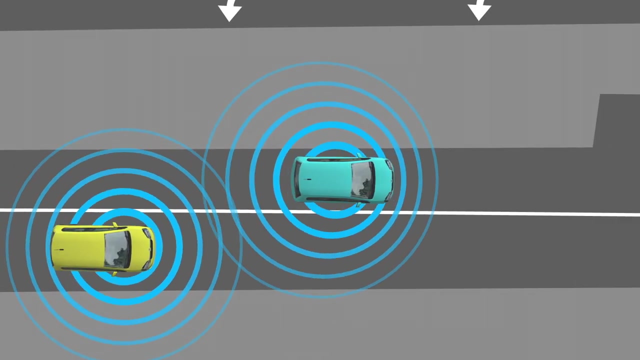 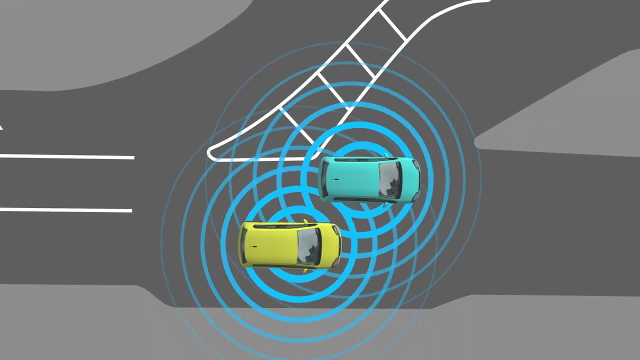 improving traffic flow and saving travelers even more time and money. With the addition of roadside units, direct communication with vehicles becomes possible, providing instant traffic notifications like red light wait times, And with onboard units installed in vehicles, the possibilities are even greater, as vehicles could then communicate directly with each other and the surrounding infrastructure. 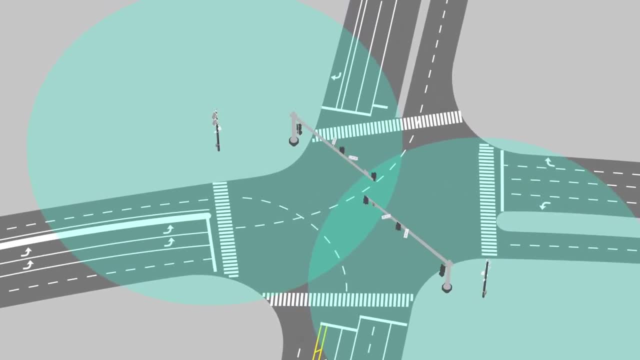 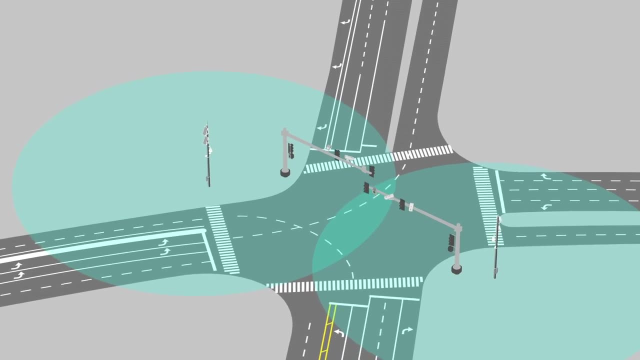 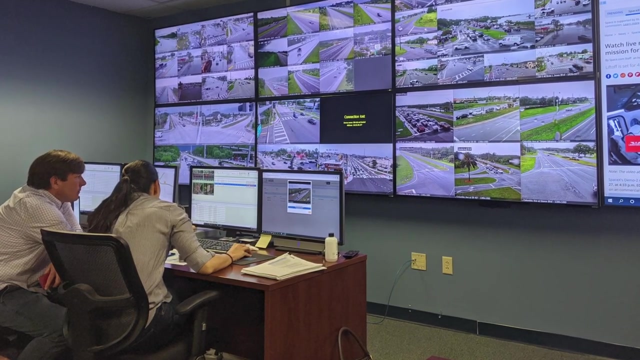 and check the speed of vehicles entering and exiting the roadway. The traffic management center now not only sees the intersection, but has much deeper traffic flow data to use for safety and roadway improvements. Speaking of traffic management centers, our new traffic management center is being envisioned as we speak. 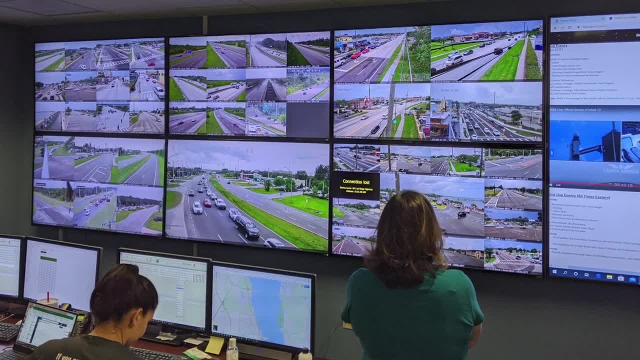 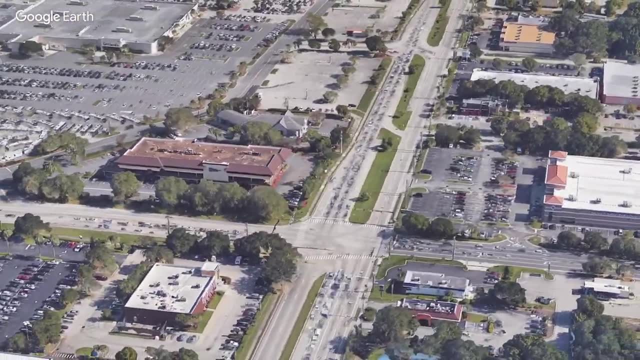 We're really excited about it. It's the brains of this entire operation, after all. Let's travel to another location and look at some more future possibilities. This is the intersection of US and Canada. It's the intersection of US 192 and Hollywood Boulevard. 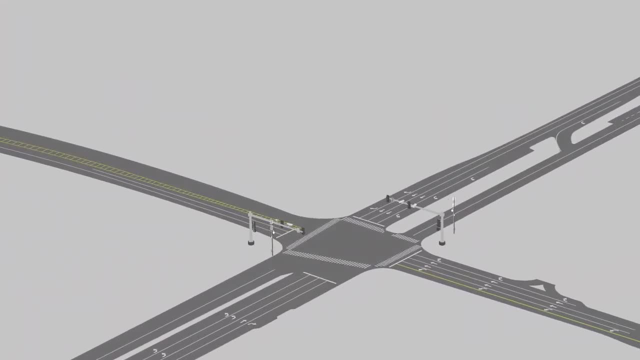 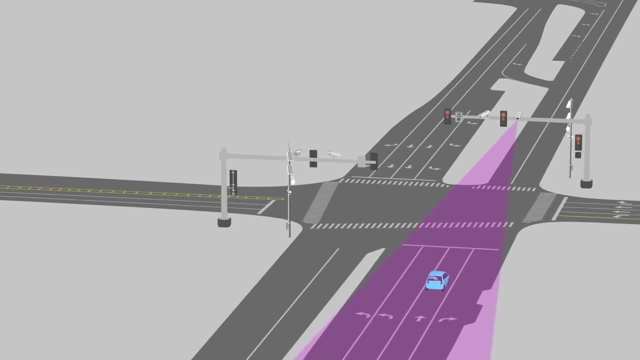 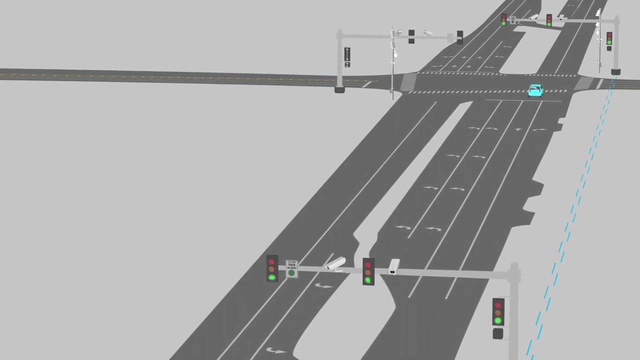 In addition to the technologies we've already seen, this intersection employs another modern technology called signal coordination. Signal coordination uses the vehicle detection sensors to allow other intersections, upstream and downstream, to communicate with each other and work together to predict traffic flow and adjust the signals. 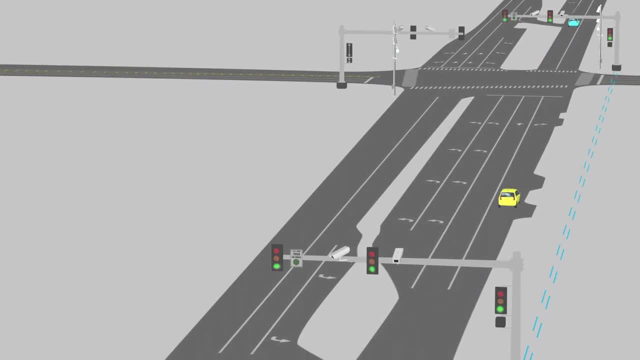 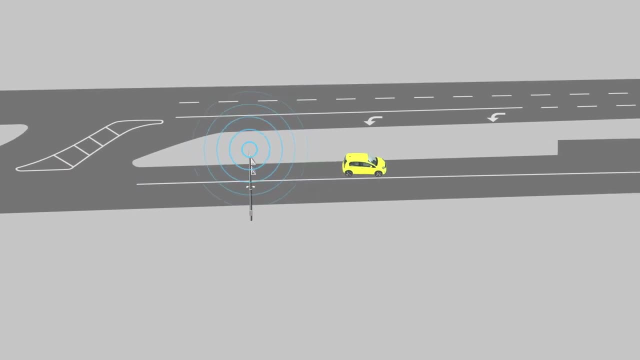 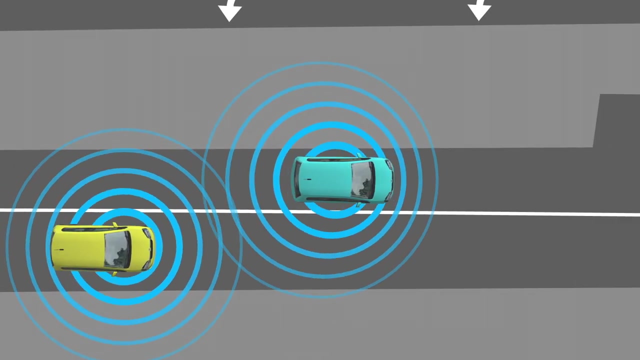 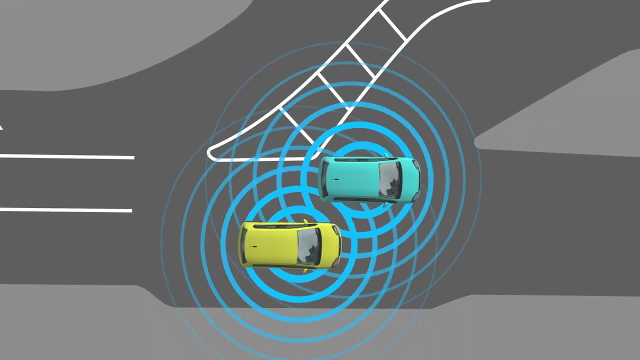 improving traffic flow and saving travelers even more time and money. With the addition of roadside units, direct communication with vehicles becomes possible, providing instant traffic notifications like red light wait times, And with onboard units installed in vehicles, the possibilities are even greater, as vehicles could then communicate directly with each other and the surrounding infrastructure. 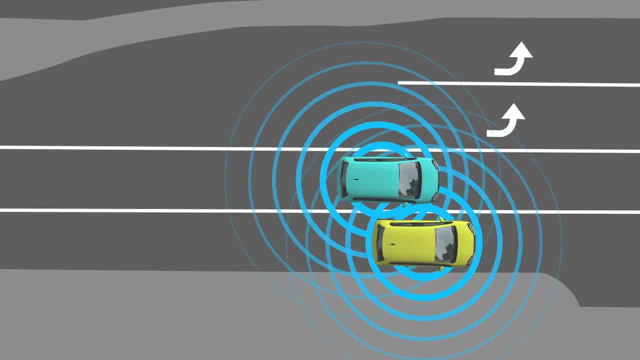 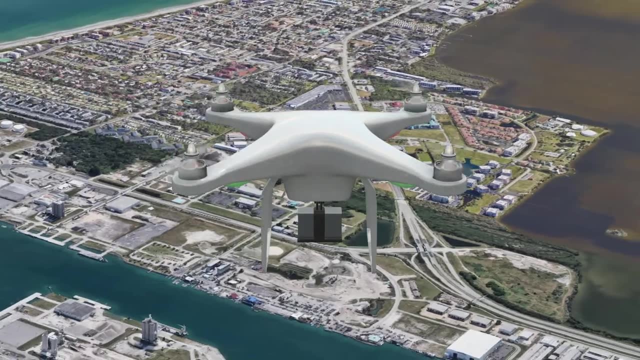 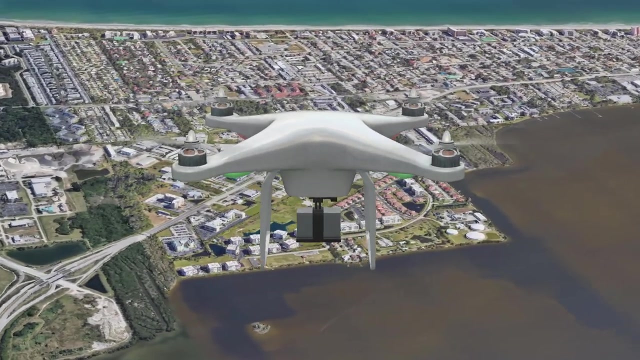 increasing travel efficiency, safety and, hopefully, less road rage. And, of course, high above the hustle and bustle, next generation drones could not only ferry our online purchases, but provide first responders, a bird's eye view of accidents, or even provide updates to your smartphone about foot traffic at a concert, festival or rocket launch. 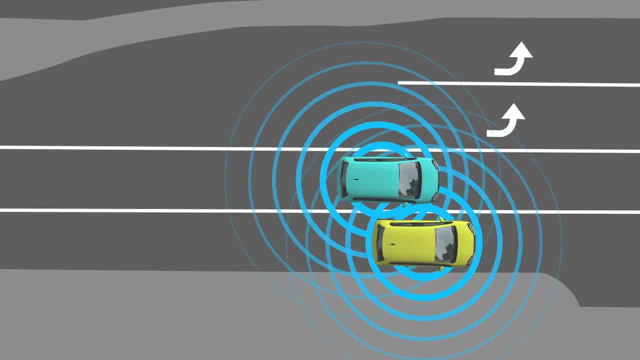 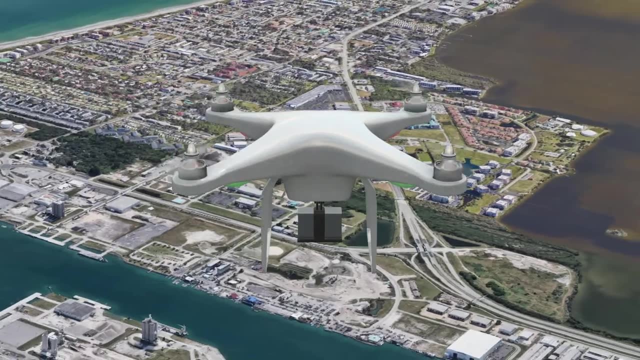 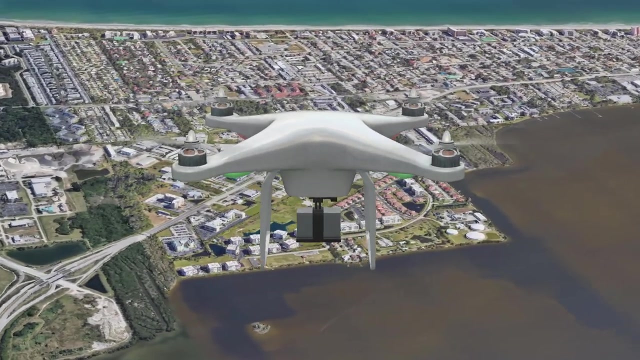 increasing travel efficiency, safety and, hopefully, less road rage. And, of course, high above the hustle and bustle, next generation drones could not only ferry our online purchases, but provide first responders, a bird's eye view of accidents, or even provide updates to your smartphone about foot traffic at a concert, festival or rocket launch. 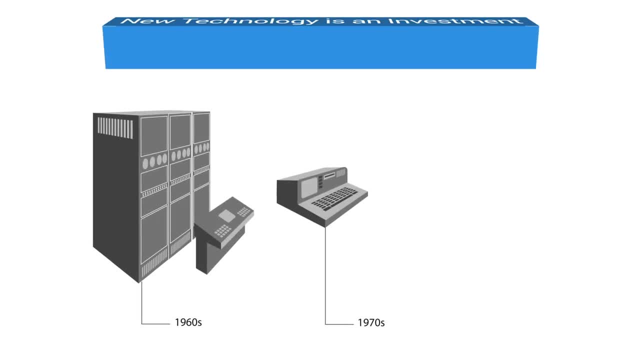 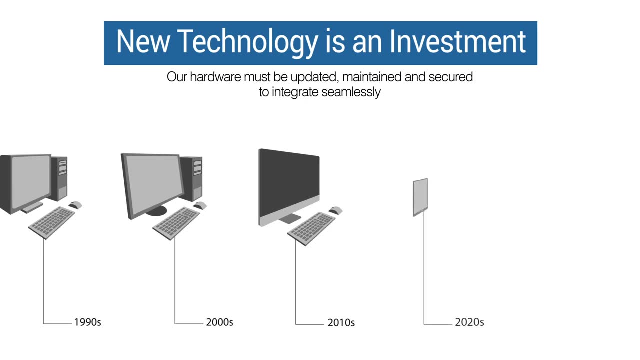 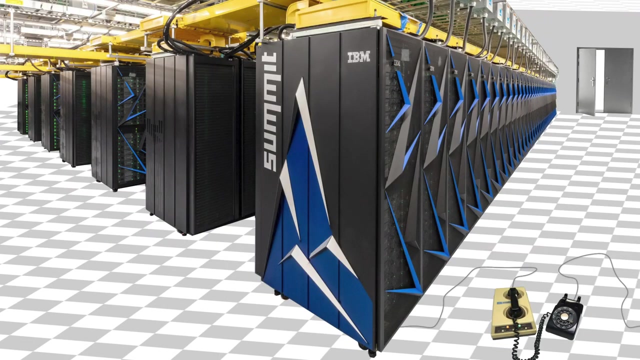 Of course, new technology is an investment. Our hardware must be updated, maintained and secured in order for future components to integrate seamlessly, in the same way that we wouldn't hook up a supercomputer to a dial-up internet connection In the present and in the future. 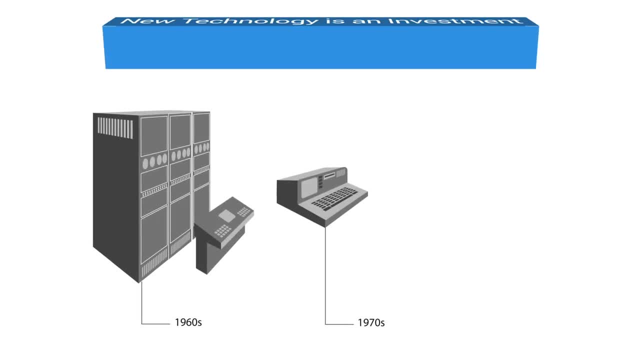 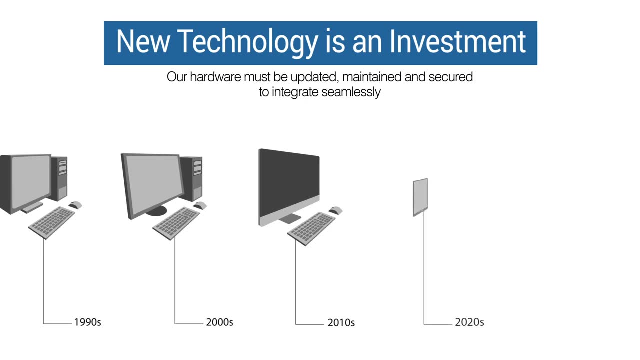 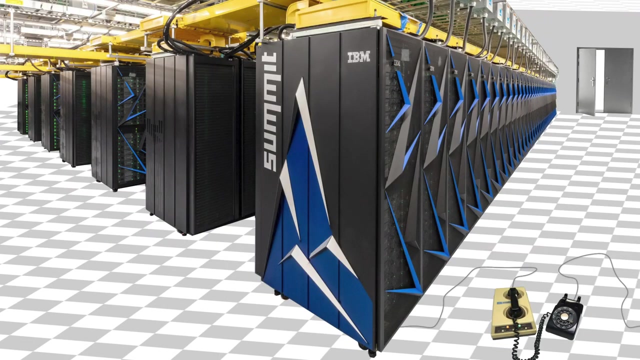 Of course, new technology is an investment. Our hardware must be updated, maintained and secured in order for future components to integrate seamlessly, in the same way that we wouldn't hook up a supercomputer to a dial-up internet connection In the present and in the future.